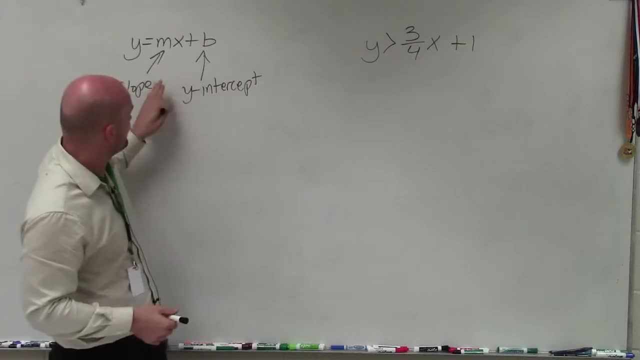 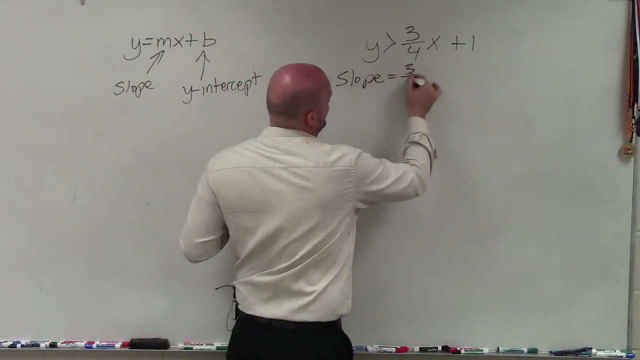 what exactly is my y-intercept? Well, looking at slope-intercept form, you can see that slope represents the coefficient of the x, which in this case we can say: my slope is equal to 3 fourths and my y-intercept is equal to my constant, which is equal to 1.. 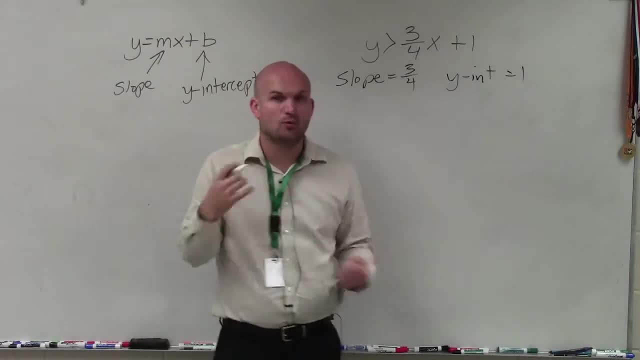 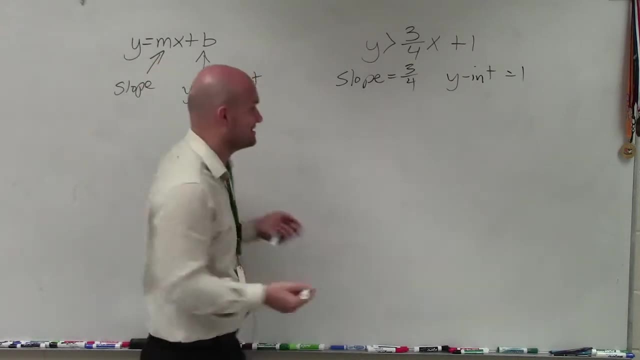 Now understand that the slope represents a ratio between the change in the y and the x coordinates between any two points, and the y-intercept represents a coordinate point, which is where the graph crosses the y axis. So to graph this I need to first graph my 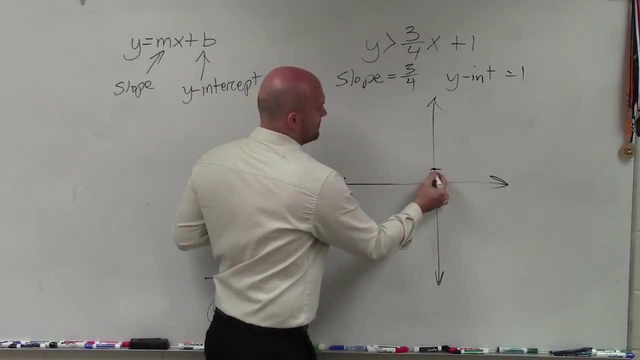 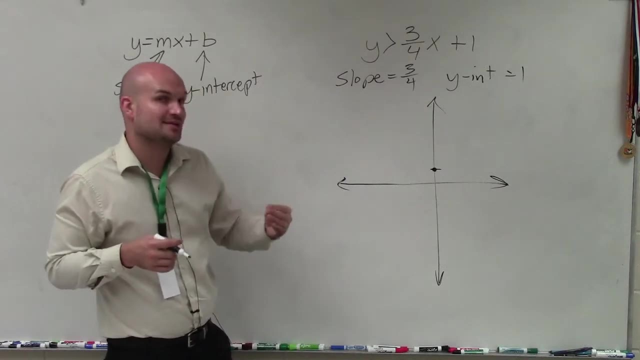 y-intercept, which is at one comma zero. I'm sorry, zero comma one. Zero comma one one. And now to apply the slope. remember, the slope represents the change in the y-coordinates between any two points over the change in the x-coordinates between any two points. 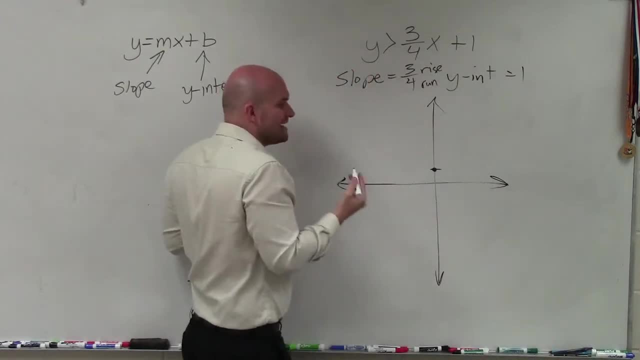 also a lot of times referred to as the rise over run. So to find my next point that lies on the line, I can use the slope. So if the change in the y-coordinates is 3, that means to find the next point, I can go up 3.. And then to change the x-coordinates to positive. 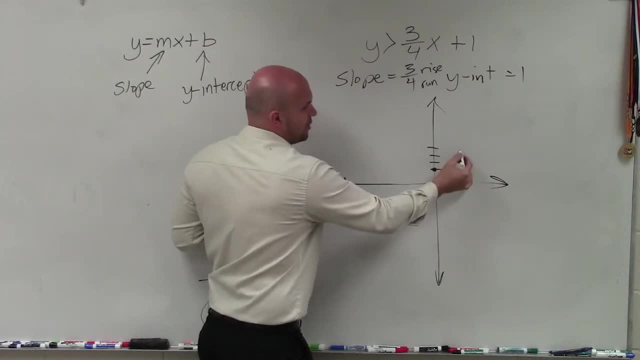 4,. I can go over 4 units, So I go up 3, over 4.. And now I have found my next point. Now, before I go ahead and graph my line, also understand that negative 3 over negative 4. 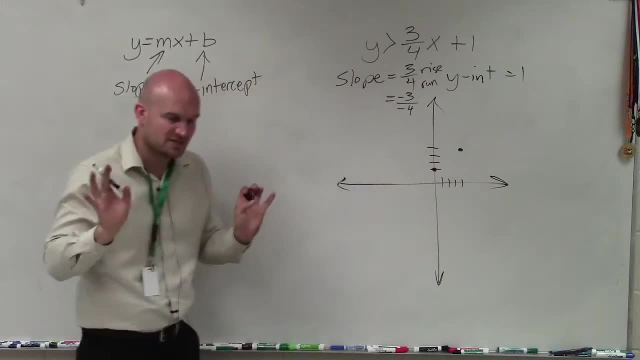 is equivalent to 3 over 4, so I could have gone down 3, left 4.. Just FYI. The next thing is now to be able to identify: is my line going to be a part of my solution or not, Is it? 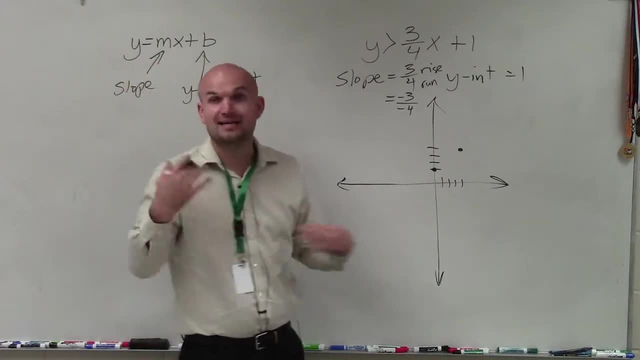 going to be dashed or solid. If it's dashed, it's not a part of the solution. If it's solid, it is So to determine that we look at our inequality symbol And since my inequality symbol is greater than not greater than, it's going to be a part of my solution. So 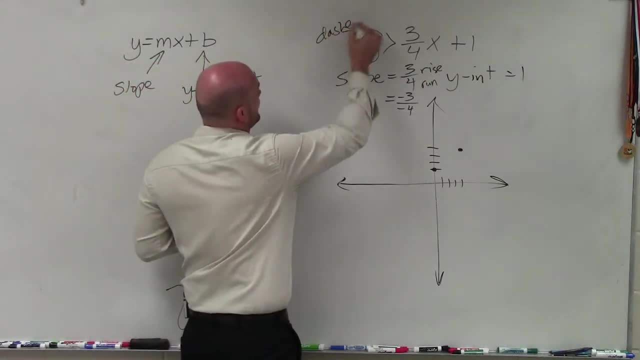 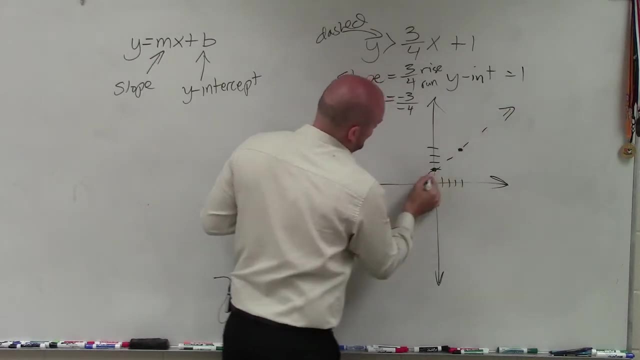 if it's greater than or equal to. I know I'm going to be using a dashed line. If it was less than or equal to, or greater than or equal to, you're going to have solid, So I'm just going to go ahead and graph my dashed line here. Okay, So now the next step: that